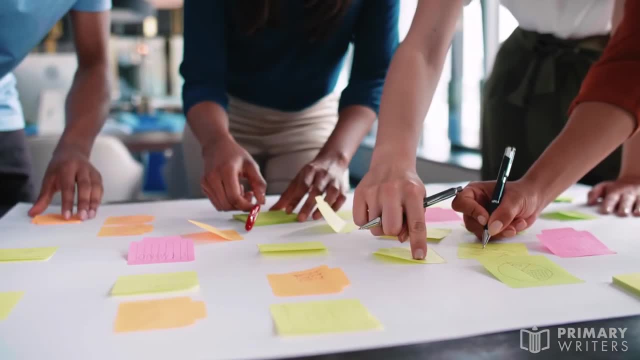 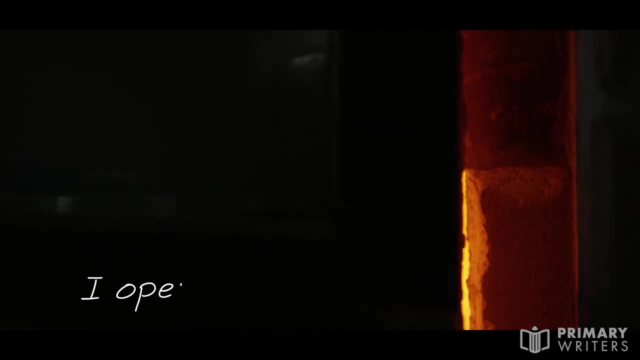 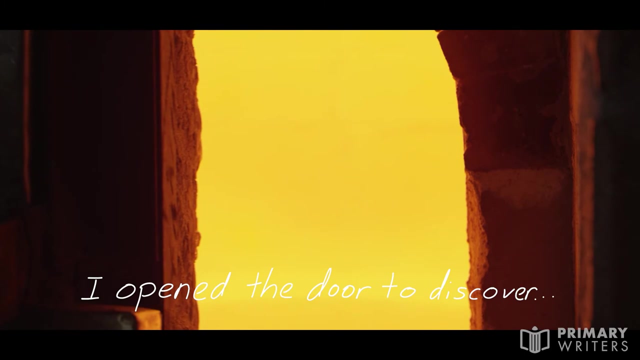 are endless. Your job is to come up with as many ideas as you can. Now, this is a timed activity and you'll have exactly five minutes. I opened the door to discover Good luck. primary writers. Your time starts now. Subtitles by the Amaraorg community. 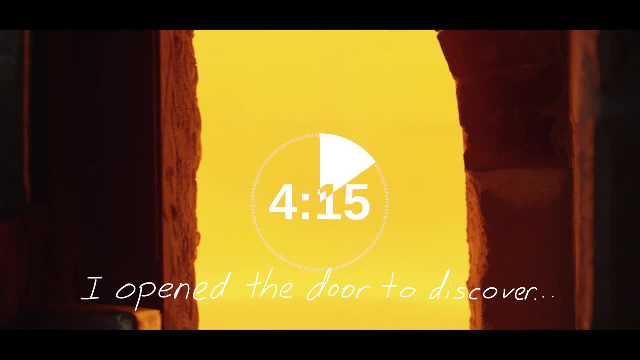